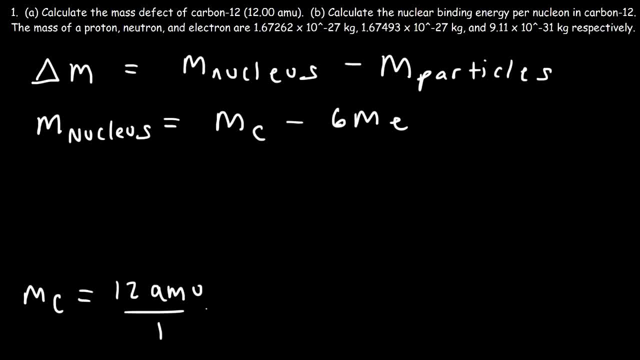 12 atomic mass units And you need to know that 1 atomic mass unit is 1.66054 times 10 to the negative 27 kilograms. And you can look that up in the internet. It's not hard to find, Just type in amu to kilograms in Google or something and it should come up. 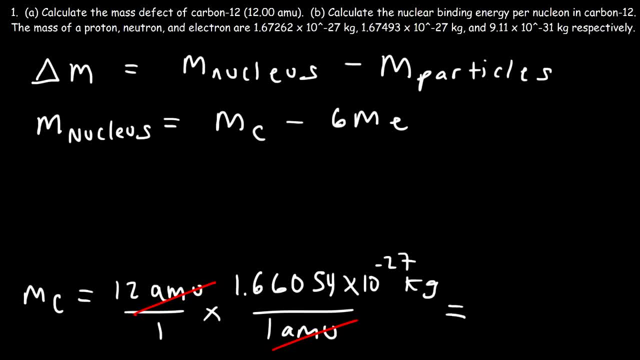 Now let's go ahead and multiply those two numbers: 1 atomic mass units, 12 atomic mass units. So the mass of carbon in kilograms is 1.99265 times 10, to the negative 26 kilograms And then minus 6.. 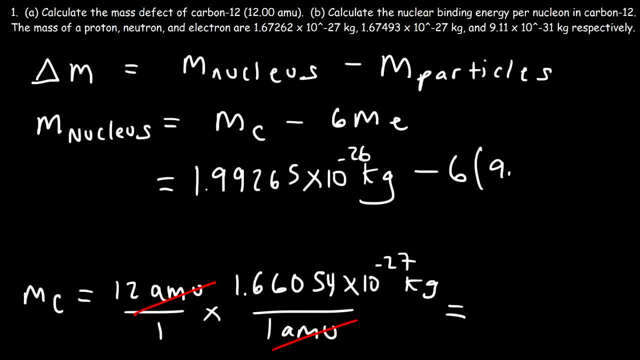 Now the mass of the electron in kilograms is 9.11 times 10 to the negative 31 kilograms. Okay, So let's go ahead and plug this in. So the mass of the carbon nucleus is 1.99210 times 10 to the negative 26 kilograms. 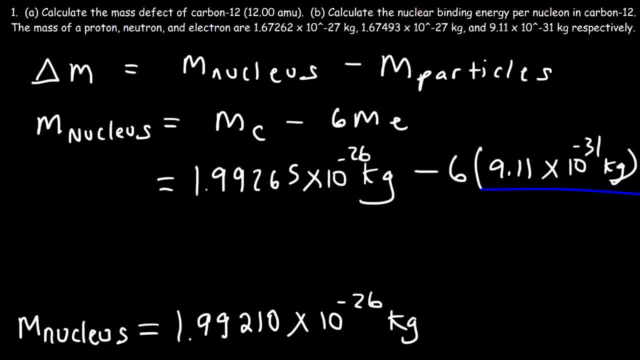 So notice that the mass of the electron is relatively insignificant. If you look at the difference between these two numbers, they're almost the same: 1.99265 versus 1.99210.. So let's say, if you decide to neglect this value, your answer shouldn't change too much. 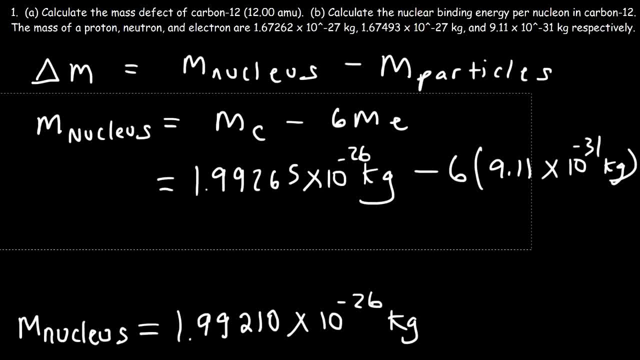 But if you want to get the exact answer, subtract the mass of the carbon atom by the number of electrons present. So now that we have that, let's get the other stuff, the mass of the particles. So we said that carbon-12 has 6 protons and 6 neutrons. 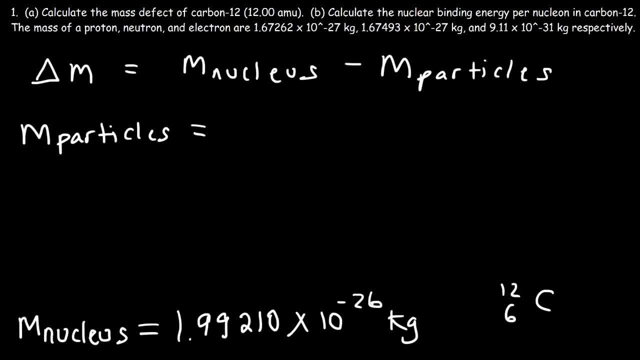 So the mass of the particles is going to be 6 mp, 6 protons and 6 mn for neutrons. So we have the mass of a proton here it is. So that's 1.674.. 262 times 10 to the negative 27,. a lot of numbers to write down. 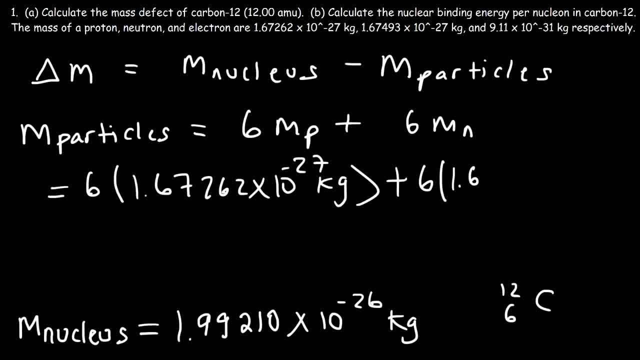 And then we have the mass of a neutron, which is a little bit heavier than a proton, but it's almost the same. Alright, so let's figure out what that's going to be. So let's do that. Okay, So let's do that. 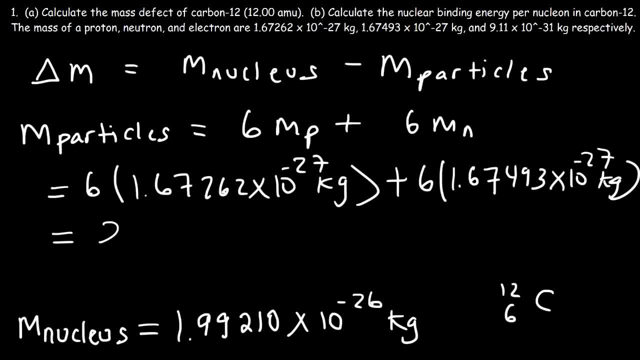 Okay. So if I typed in everything correctly, this is what I got: 2.00853 times 10 to the negative 26 kilograms. So hopefully you got that too. So now we can calculate the mass defect. So the mass of the nucleus, that's 1.9921 times 10 to the negative 26 kilograms. 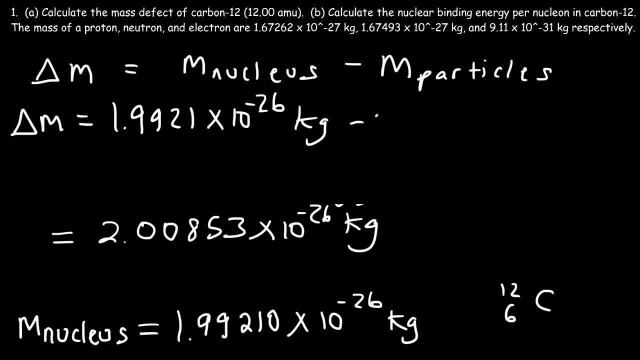 Okay, And then the mass of the individual particles that make up the nucleus is this number, And so let's see what this is going to be. So this is going to be negative 1.674 times 10 to the negative 26 kilograms. 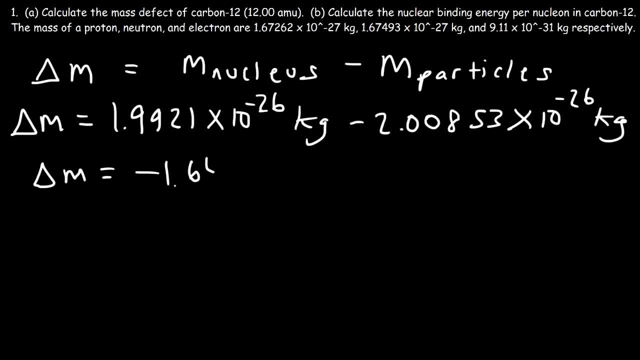 Okay, So this is going to be negative 1.674 times 10 to the negative 26 kilograms. Okay, So this is going to be negative 1.674 times 10 to the negative 28 kilograms. So that's the difference between the mass of the carbon nucleus and the mass of the. 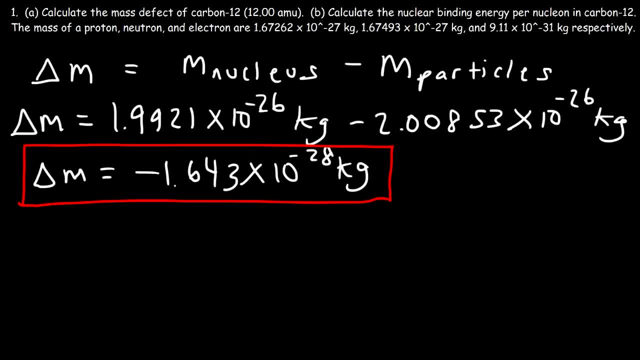 individual subatomic particles that make up the nucleus. So that's the mass defect of carbon 12.. Now let's calculate the nuclear binding energy per nucleon. So we need to use this equation: Delta E is equal to delta C minus. 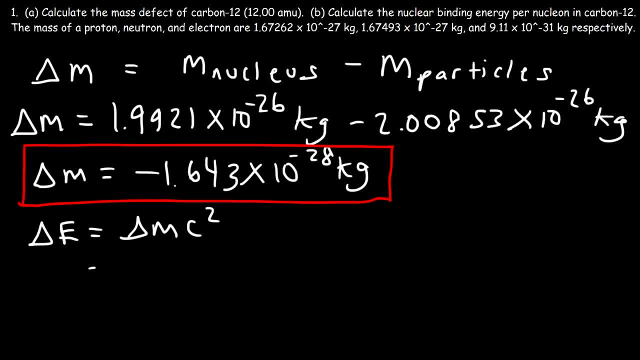 is equal to delta, m, c squared. So the mass defect is this number: C represents the speed of light, which is 3 times 10 to the 8 meters per second, and then we have to square that number, So the change in energy is negative 1.4787 times 10 to the negative 11 joules per individual. 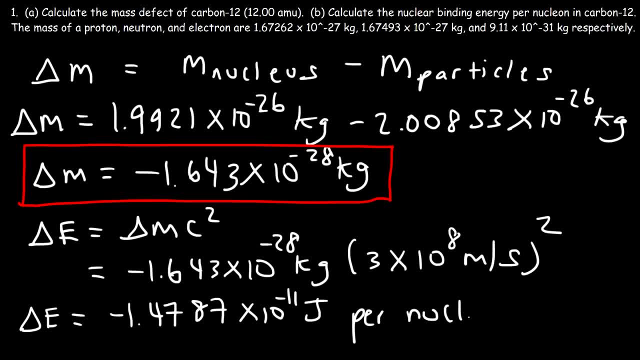 nucleus. Now you might be wondering: why is this answer negative? Now, what this means is that if you take the 6 protons and the 6 neutrons and put them together to form the carbon nucleus, Energy will be released, since mass is lost. 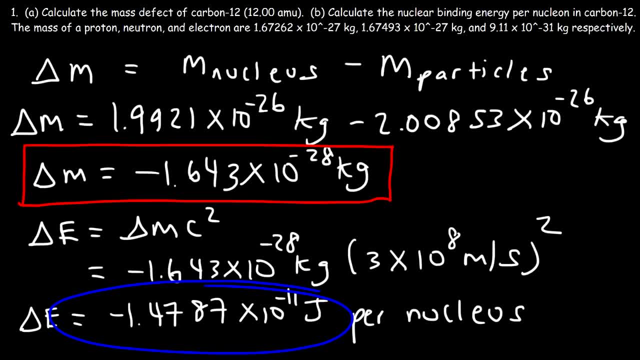 So what really happens is the mass is converted to energy. So, as those 6 protons and 6 neutrons come together to form the nucleus, that change in mass, that difference in mass, was converted into the energy that was released by that. 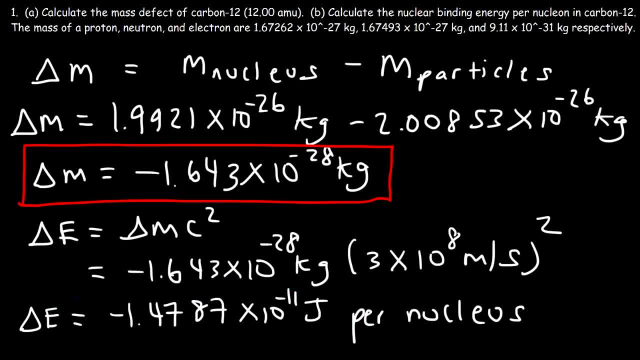 process. So that's why it's negative. Now the reverse is positive. Let's say, if you have a carbon nucleus, It's going to take this much energy To break the nucleus into its individual particles. So the sign depends on what you're trying to do. 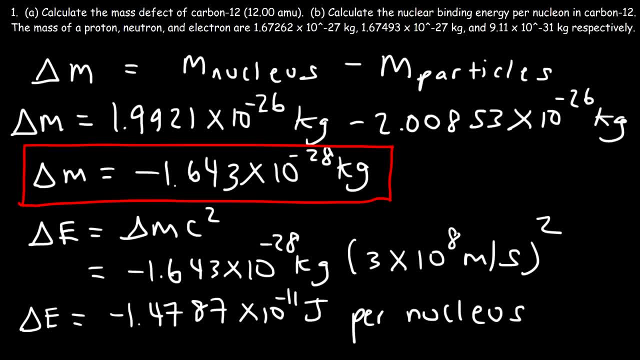 If you're trying to bring the particles together to make up a nucleus, then energy will be released. Delta E will be negative. If you're trying to put in energy to break up the nucleus into its individual particles, then Delta E is positive. 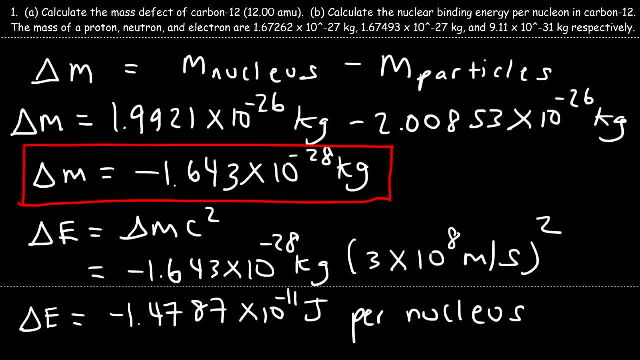 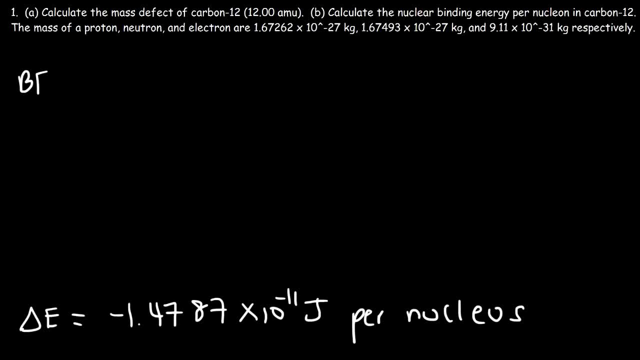 Now to calculate the binding energy, the energy that we need to break the nucleus. that's going to be a positive value. So we need to calculate the binding energy per nucleon. Now you need to know what a nucleon is. What do you think a nucleon is? 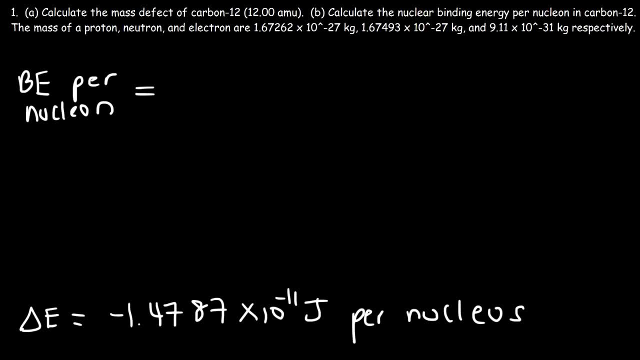 A nucleon is basically a particle in the nucleus, So protons and neutrons are considered to be nucleons, not electrons. So carbon 12 has 6 protons and 6 neutrons. So 6 plus 6 is 12.. 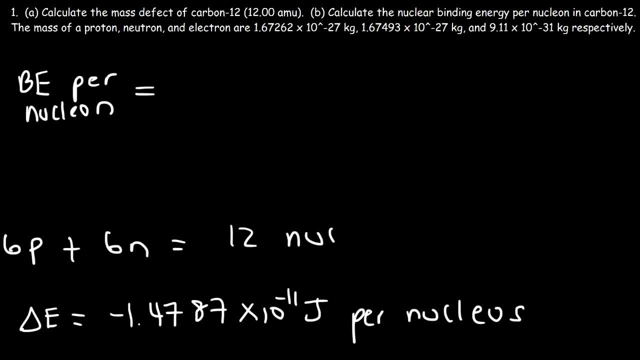 So we can say that it has 12 nucleons. So to calculate the binding energy per nucleon, the nuclear binding energy, it's going to be this value. Well, let me convert it. So let's start with this number. This is the energy per nucleus. 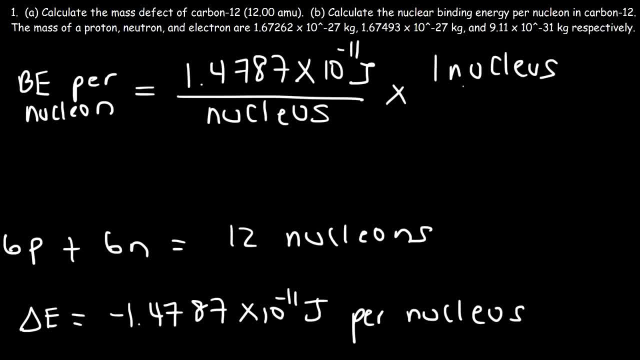 And one carbon 12 nucleus. How many neutrons? 7.. How many neutrons? 7. 5., 6., 6., 5. 1. 1., 1., 1., 1. 1.. 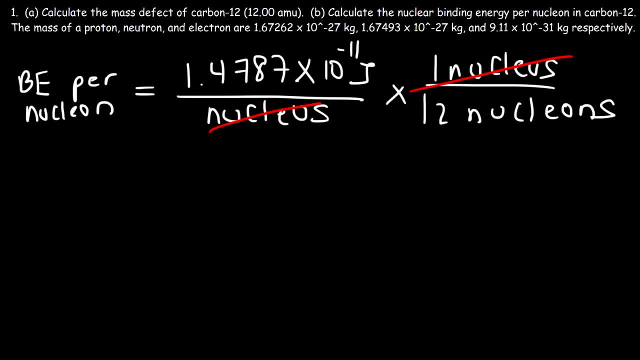 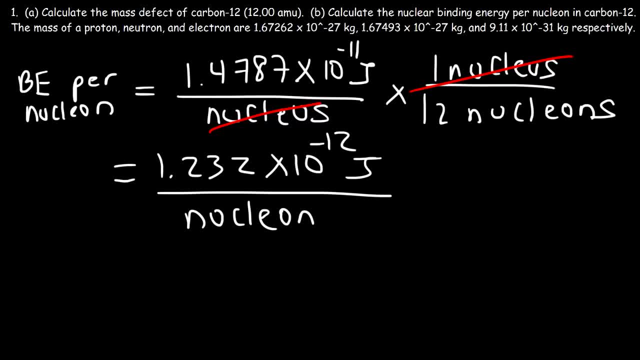 nucleon. Now sometimes you may need to report your answer in mega electron volts per nucleon. If you need to do that, you can use this conversion. One mega electron volt is 1.6 times 10 to the negative 13 joules. 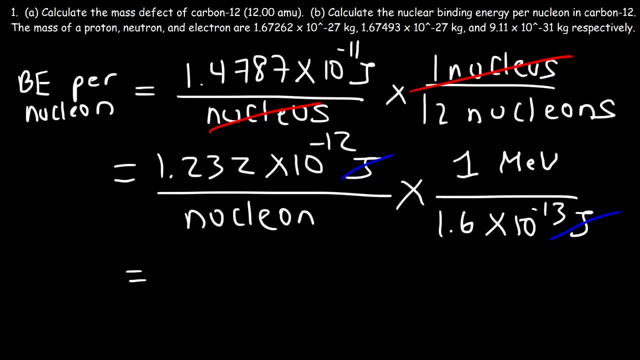 So the unit joules will cancel, and let's go ahead and divide these two numbers So you should get 7.7 mega electron volt per nucleon. So that is the nuclear binding energy of carbon-12.. That's all you need to do. 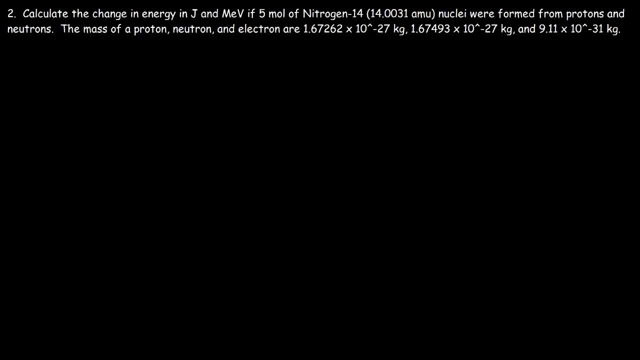 Number two: Calculate the change in energy in joules and mega electron volts if five moles of nitrogen-14 nuclei were formed from protons and neutrons. So if you want to try this problem, feel free to pause the video and work on it. 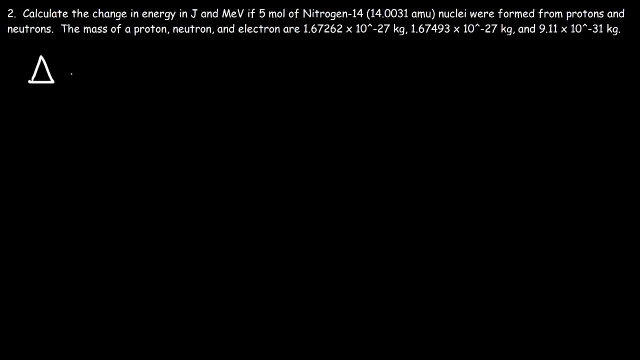 So let's begin. So we said that the mass defect is the difference between the mass of the nucleus and the mass of thease nucleus, particles that make up the nucleus. so in this case we're combining protons and neutrons to make up the nitrogen nuclei, and so energy is going to be released. 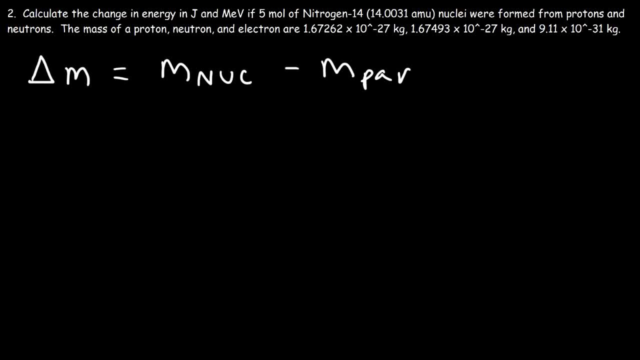 when that happens, anytime a bond is formed between two atoms or two particles, energy is released, so we should expect a negative energy value for our answer. now let's calculate the mass of the nucleus first. so it's going to be the mass of the nitrogen atom minus the seven electrons that are in. 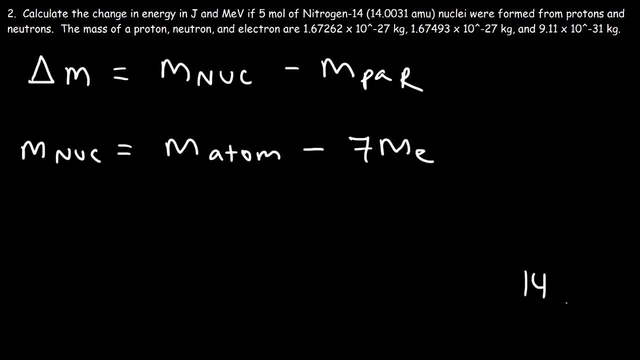 the nitrogen cloud. now, keep in mind: nitrogen 14 has an atomic number of 7, so it has seven protons, seven neutrons and also seven electrons. the number of neutrons is going to be 14 minus 7 and for an atom, the protons and electrons are the same. if the atom is. 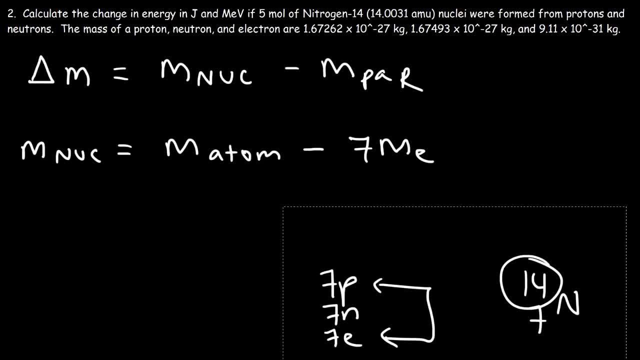 electrically neutral, which by definition it is. now let's calculate the mass of the nitrogen atom. so we're given the massive atomic mass units. so that's 14.0031 amu. you know, based on the last problem, we know that one atomic mass mass unit is 1.6605, 4 times 10, to the negative 27 kilograms. so that's not. 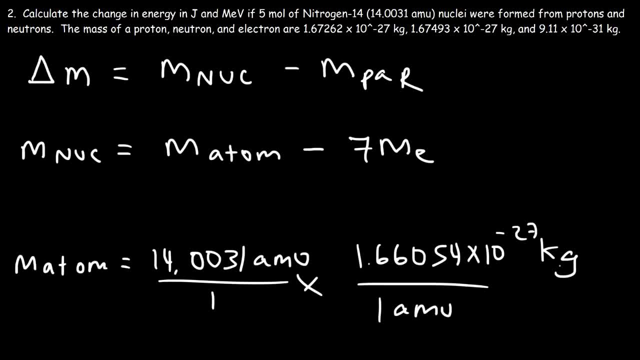 going to change, and so the mass of the nitrogen atom is 2.325, 27 times 10 to the negative 26 kilograms, and then the mass of the electron is 9.11 times 10 to the minus 31 kilograms. so let's go ahead and plug that in. 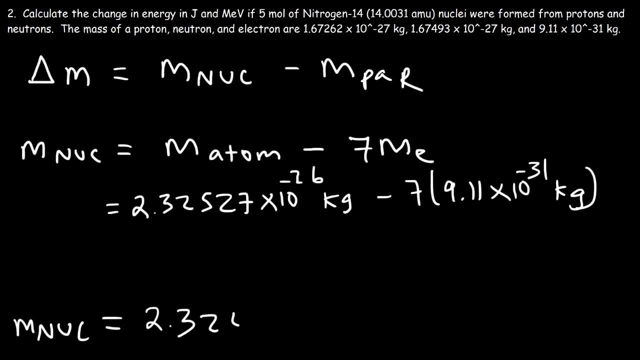 so you should get 2.32463 times 10 to the negative 26 kilograms. so now we need to calculate the mass of the subatomic particles in the nucleus, and so we said that nitrogen-14 has seven protons and seven neutrons. so the mass of a proton, its 1.67262 times 10 to the negative 27. 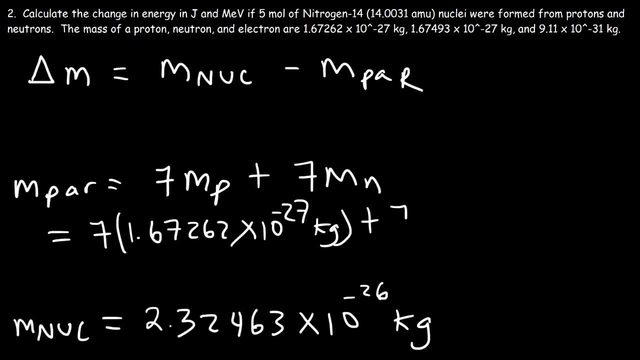 kilograms, and then the mass of a neutron is 1.67493 times 10 to the negative 27 kilograms. so you should get this number 2.34364 times 10 to the negative 26. so now let's go ahead and use this equation. so the 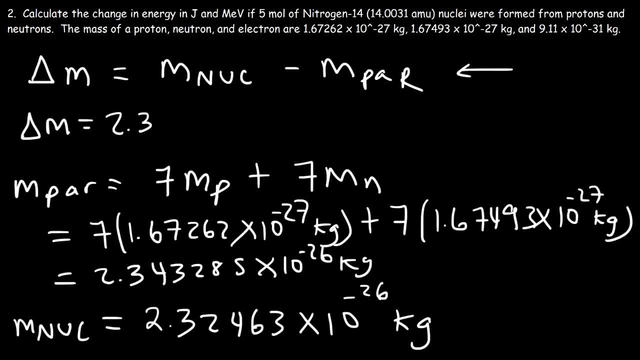 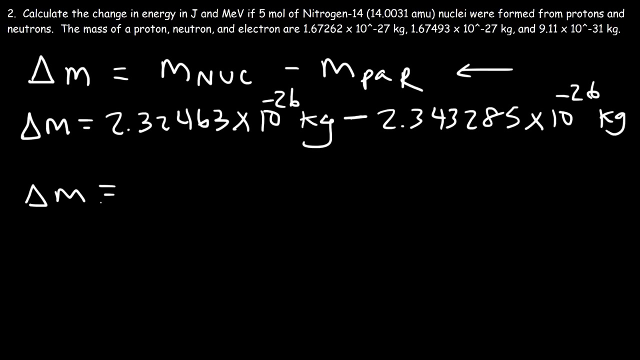 mass defect is the difference between these two numbers. So if we subtract 2.32463 times 10 to the negative 26,, by 2.343285, to the same power, we should get negative 1.8655 times 10 to the negative 28 kilograms. 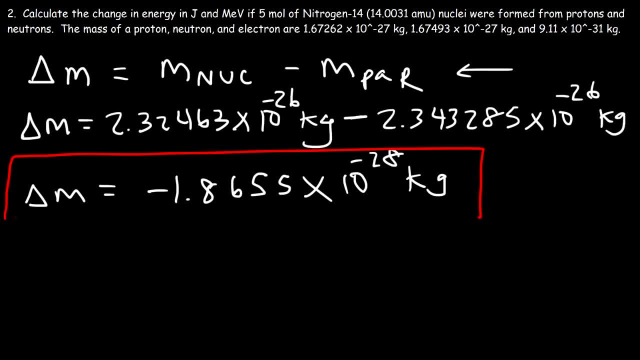 So that is the mass defect in this problem, that's the change in mass. So when the 7 protons and the 7 neutrons get together to form the nitrogen nucleus, this is how much mass is lost, And so that mass is changed into energy. 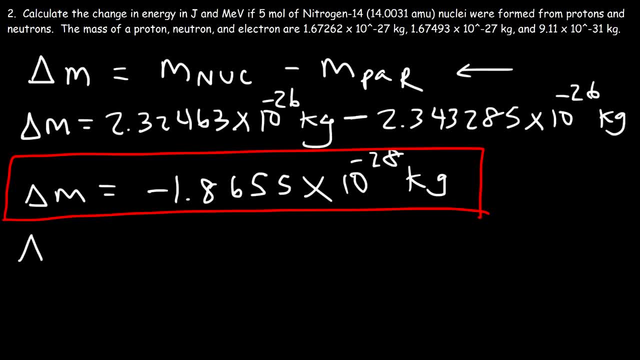 So now let's calculate how much energy is released during the process. So this is going to be negative 1.8655 times 10 to the negative 28 kilograms multiplied by the square of the speed of light. Okay, Okay. So this is 2.32463 times 10 to the negative 28 kilograms. 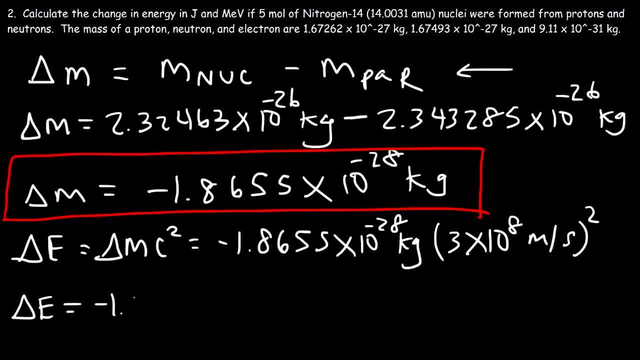 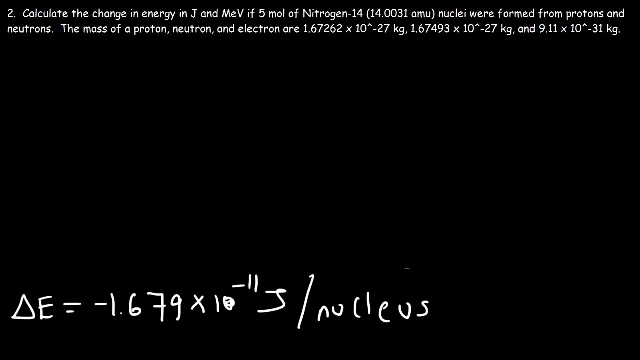 And so the change in energy is negative 1.679 times 10 to the negative 11 joules, and this is per nucleus. So that's how much energy is released if only one nucleus is formed. Okay, Okay, Okay, Okay. 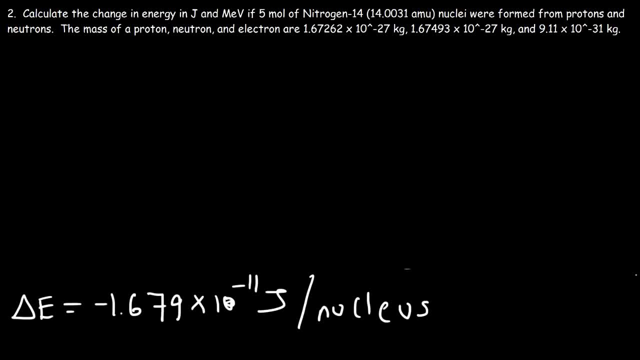 formed, how much energy would be released. let's start with five moles now. one mole is equal to Avogadro's number six point zero, two, two times 10 to the 23, and we're dealing with the nitrogen nuclei and the energy change for just one. 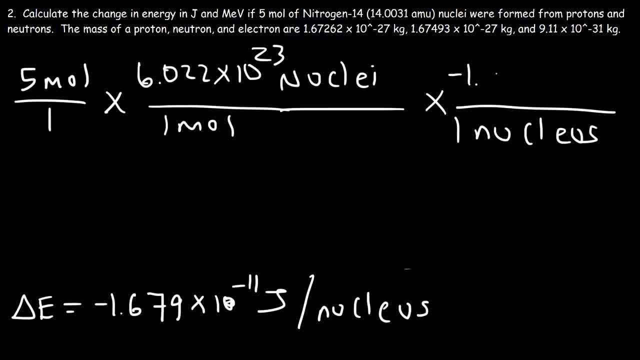 nucleus is 1.679 times 10 to the negative 11 joules, and so we could see the unit moles will cancel and the nucleus will cancel as well. so this will give us the energy change in joules if five moles of nitrogen nuclei were. 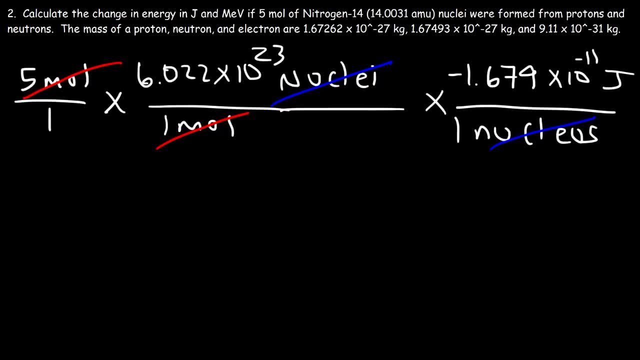 formed from protons and neutrons, and so this is equal to five point zero, five, five times 10 to the 13 joules. and so that's the answer in joules. now, if you want the answer in mega electron volts, simply convert it, divided by 1.6 times 10, to the 13 joules. 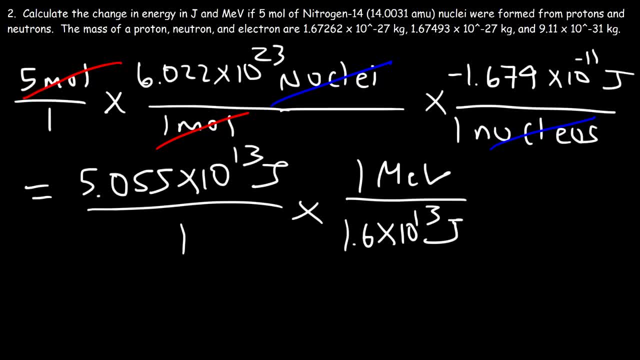 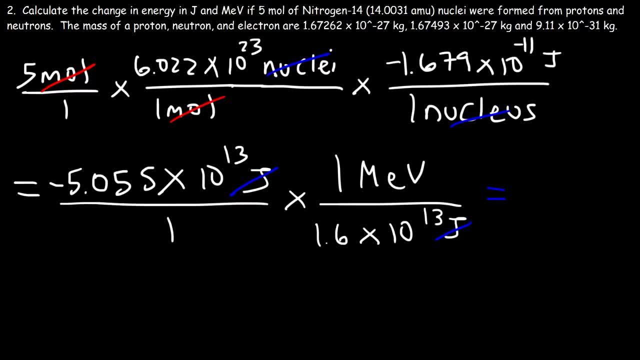 ok, that's supposed to be the answer. so if you're wondering why the sudden change in the screen, that's just me editing this video because I made it before, but I noticed that I missed a negative sign. one mega electron volt is not positive 13, but it's 1.6 times 10 to.